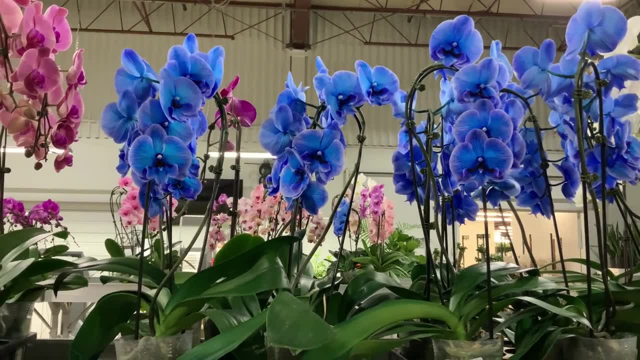 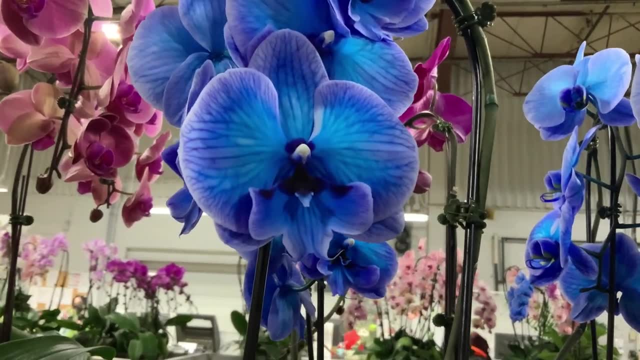 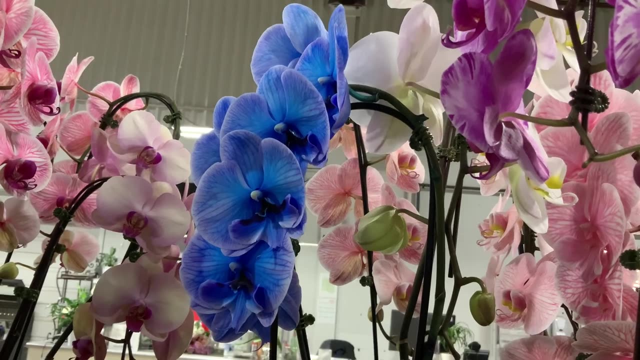 Have you ever wondered how blue orchids are made? Well, it's probably obvious that this blue orchid color is artificially created and not a result of mutation or hybridization. So what is the grower's trick to make them blue? Because orchid leaves and roots still look green. 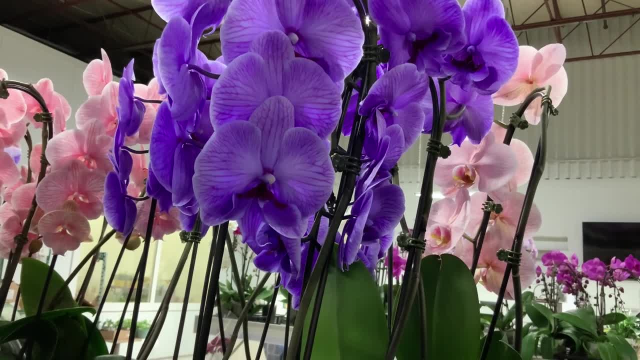 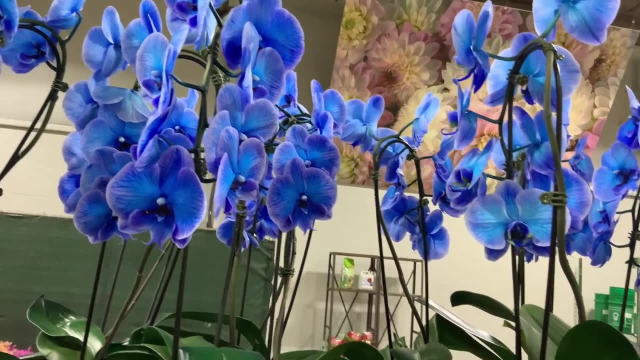 still look normal and don't have any blue pigmentation present. So if, for example, the blue dye was to be absorbed through the substrate, we would see it inside the roots, but we don't. And we know that orchids are epiphytes and they absorb moisture directly. 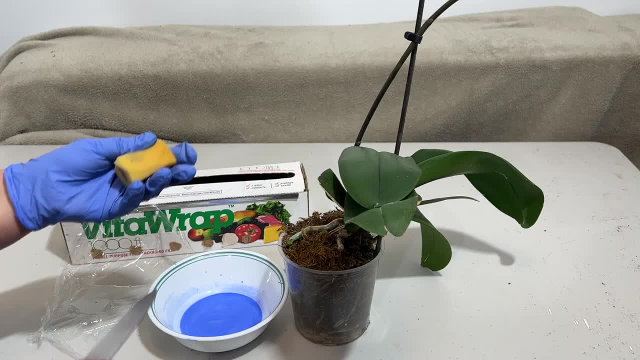 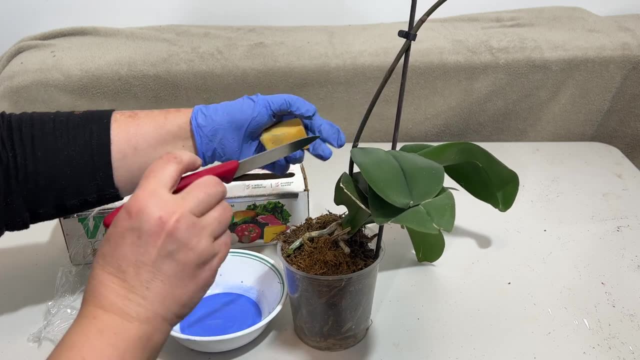 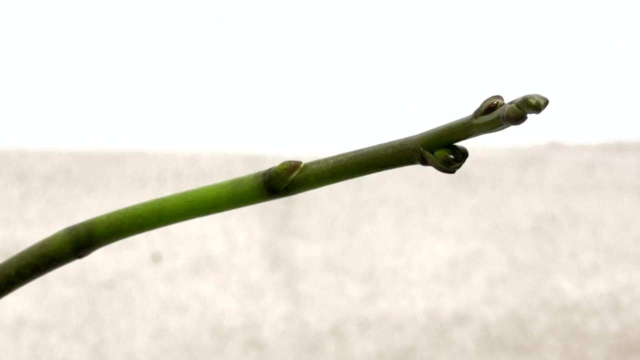 from the air through a very unique vellum and layer And I suppose that it can be a very complicated and dangerous process in order to achieve these blue flowers through the aerial root system. I can tell you that it's done through the flower spikes and it takes a lot. 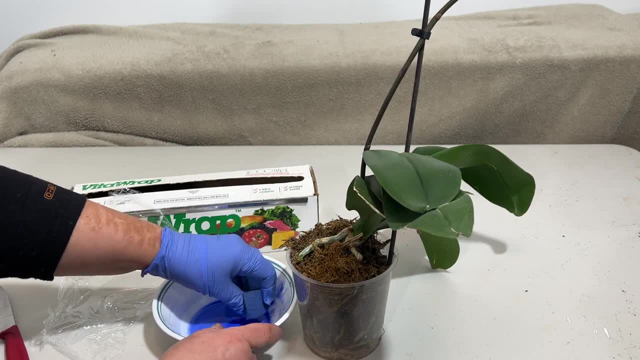 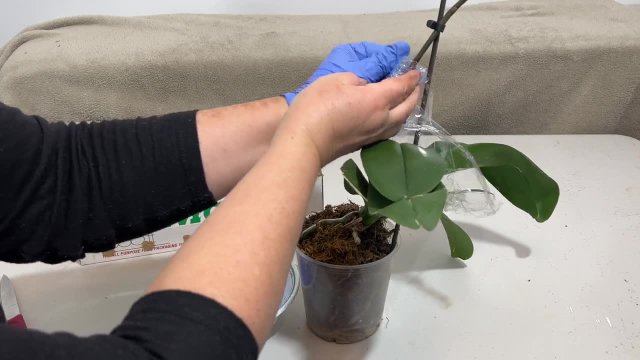 of time to do that. So, if you're a grower and you're a grower and you're a grower, because this part of the orchid grows and develops very slowly, up to two to three months from the starting point until the blooming period, blue dye can be absorbed through. 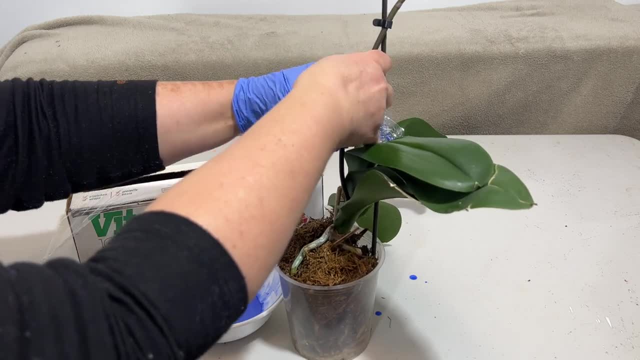 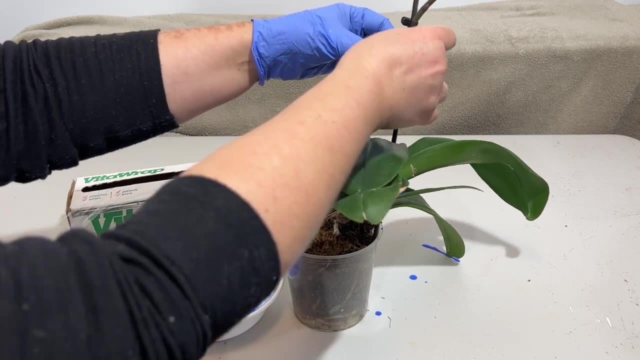 the small cuts and wounds made for this purpose on orchid flower spikes, or it can be injected directly into the vascular system of the orchid flower spikes, which is a set of conductive tissues that allow for blue dye to be delivered directly to the development of the orchid flower. 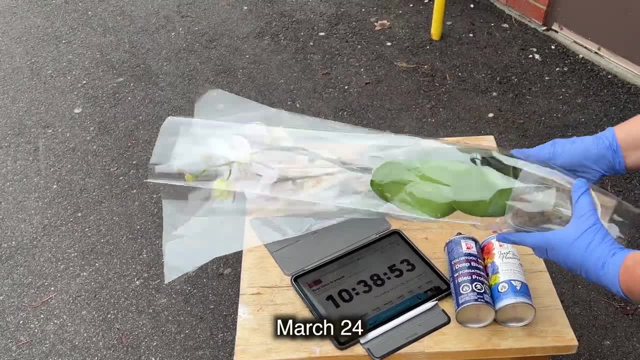 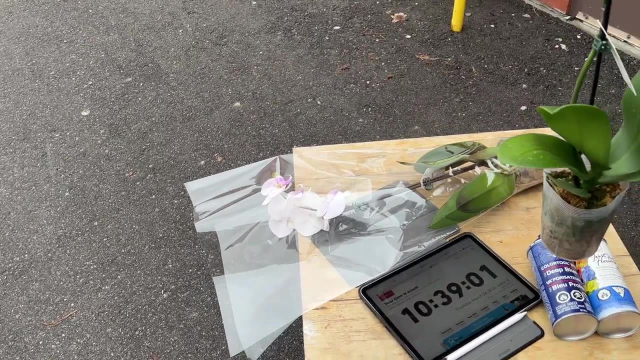 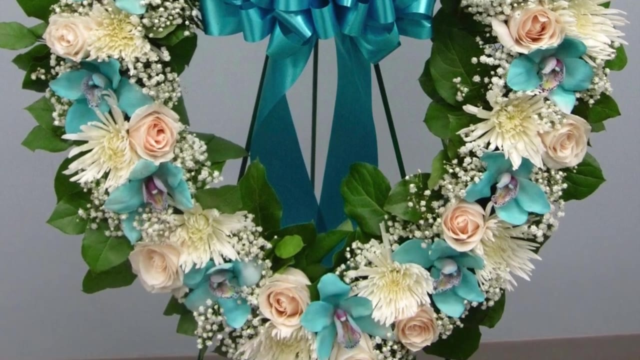 and buds. Because of this time and labor-consuming process, blue orchids are typically a lot more expensive- about 50% more expensive- in comparison to natural colors, And as a florist, you have to use these orchids for many different orders and for many different designs, And I found that. 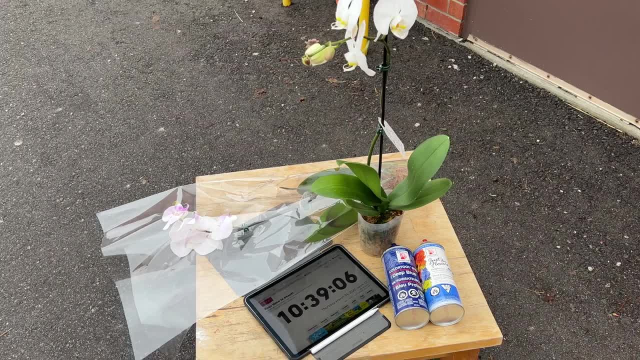 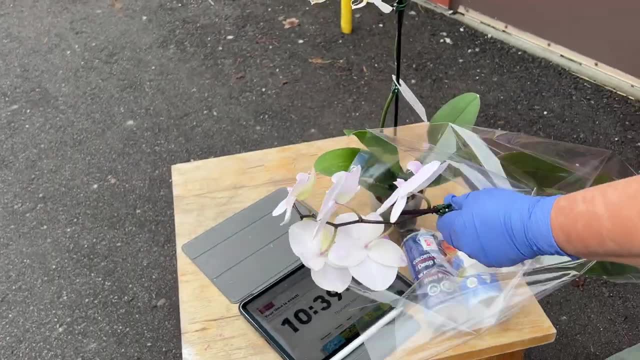 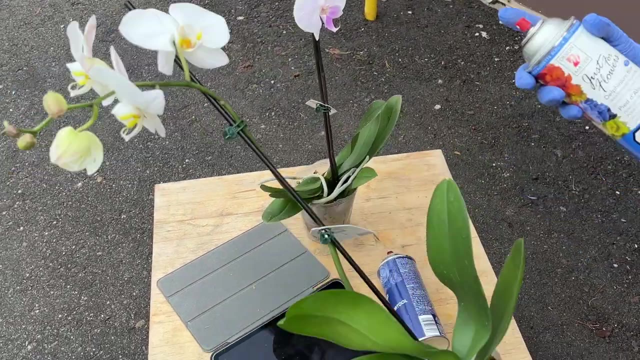 buying these blue orchids from growers, even for wholesale prices, is very expensive And I start to make them myself. It is much easier than you may think if I use a simple, affordable brand of floral spray. Some people think that the chemicals in the spray may hurt the delicate. 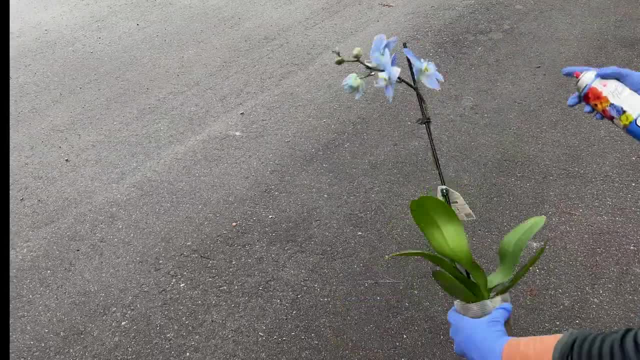 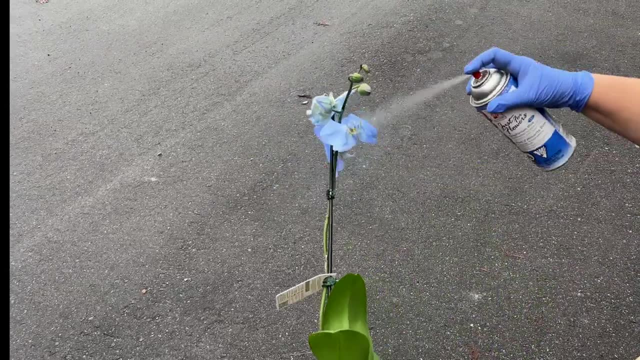 orchid flowers. And while orchid flowers may look delicate, they aren't really that delicate, And I'm conducting this experiment to prove it to you. I can make a blue orchid within just a couple of minutes. I can use any different brand of floral spray to achieve different